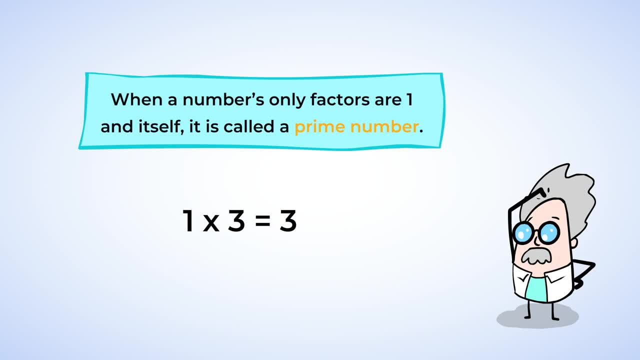 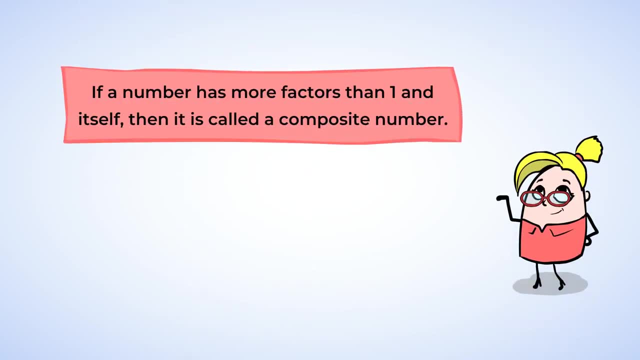 Because the only way to get a product of 5 is to multiply 1 and 5.. And if a number has more factors than 1 and itself, then it's called a composite number. 10 is a composite number Because you can multiply 1 and 10 or 2 and 5 to get to a product of 10.. 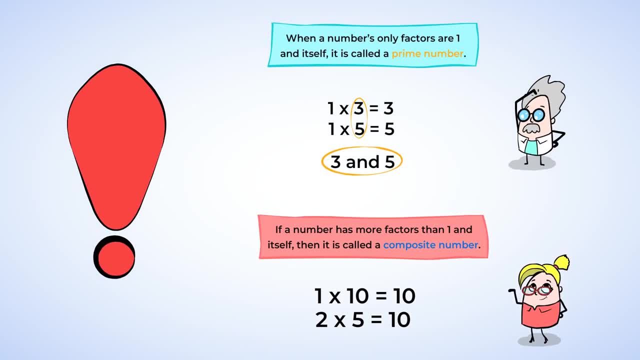 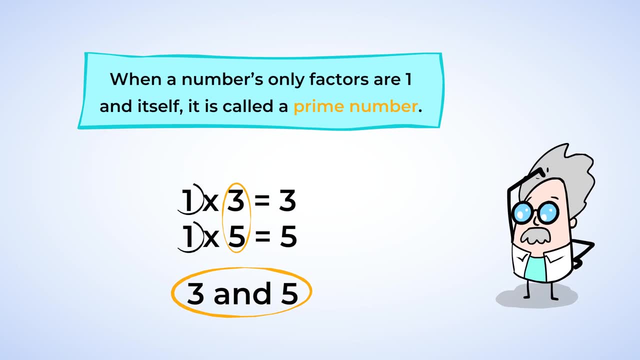 So how can we find the factors of a number? Well, a great way is to create an organized list. We always start with 1, since all numbers have 1 as a factor, And then we work our way up to the number itself. 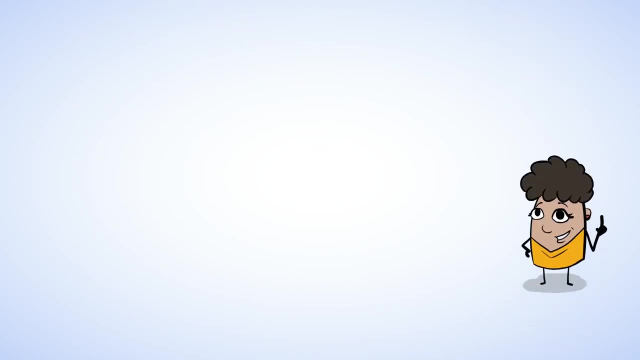 So let's try this out. Let's find all the factors of 20.. Okay, we're going to start with 1.. 1 multiplied by 20 is equal to- That's right- 20.. Next we move on to 2.. 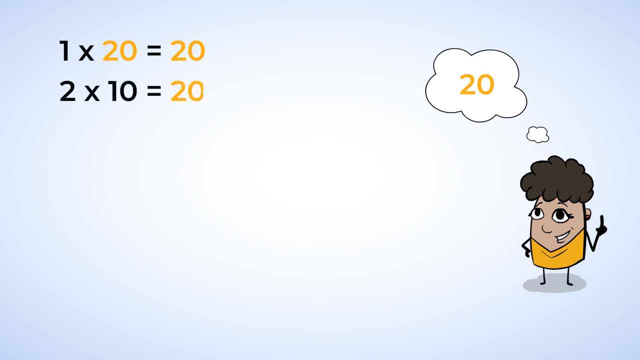 2 multiplied by 10 is equal to 20.. Next 3.. Oh, There's nothing that we can multiply by 3 to get to 20.. When we skip count by 3s, it goes from 18 to 21.. 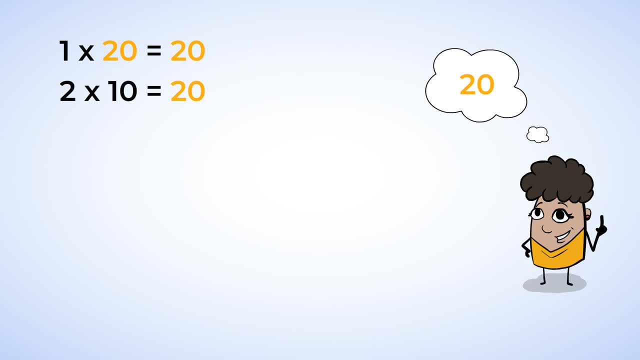 And so 3 isn't a factor, It's a factor of 20.. Moving on to 4.. 4 multiplied by 5., That's equal to 20.. And after 4 comes 5.. Ew wait, Look, we already found that 5 is a factor. 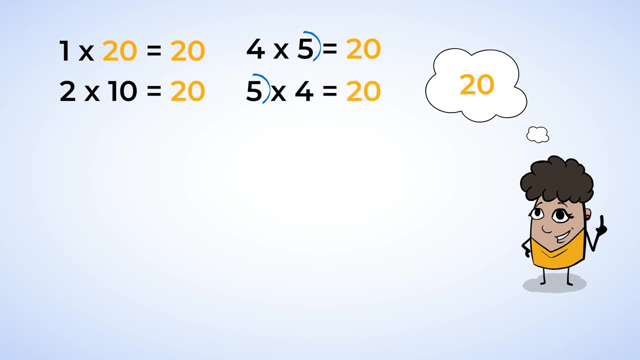 And hey, this means we've found all the factors of 20.. Great job. So far, we've seen a couple of numbers that have 2 as a factor. Both 6 and 20 have factors of 2. And this is because 6 and 20.. 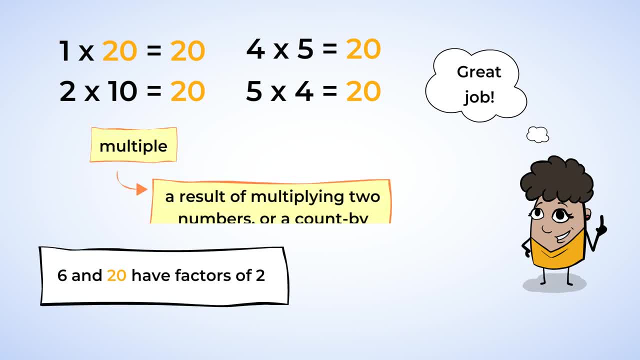 are multiples of 2.. A multiple is a result of multiplying 2 numbers or a count by. When you skip count, you are listing all of the multiples of the number you are skipping by 2,, 4,, 6,, 8,, 10.. 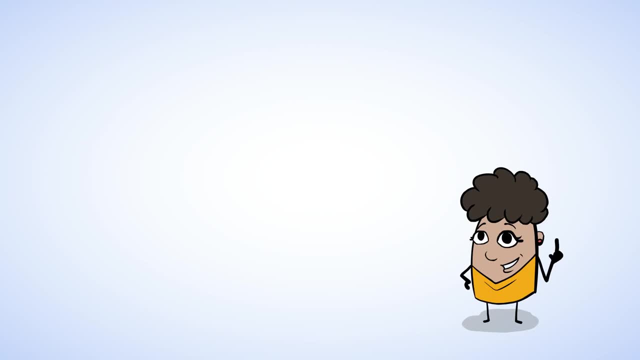 These are all multiples of 2.. I bet you can keep it going. Let's try this problem and find the first 5 multiples of 4.. All right, we can do this. Let's skip count by 4.. Okay, 4,, 8,, 12,, 16,, 20.. 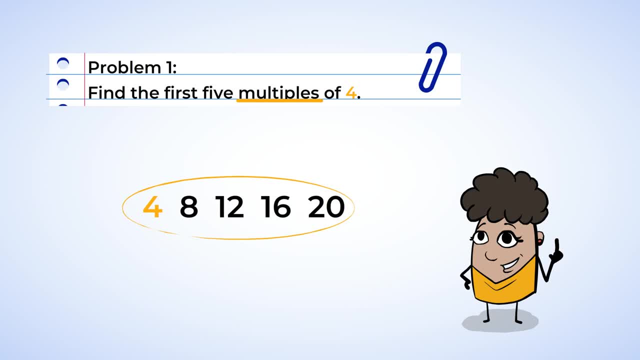 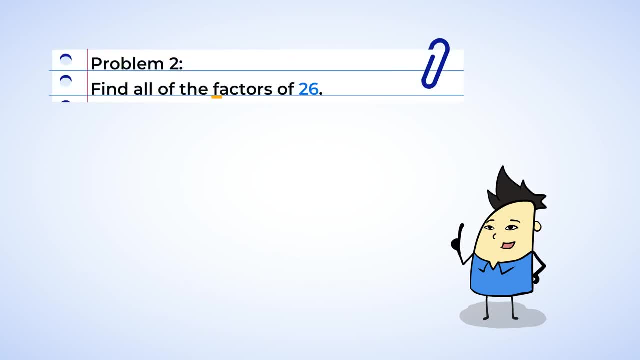 Excellent, You just found the first 5 multiples of 4.. I think we can do the next one. All right, so we need to find all of the factors of 26.. Okay, we can do this. Let's start with 1.. 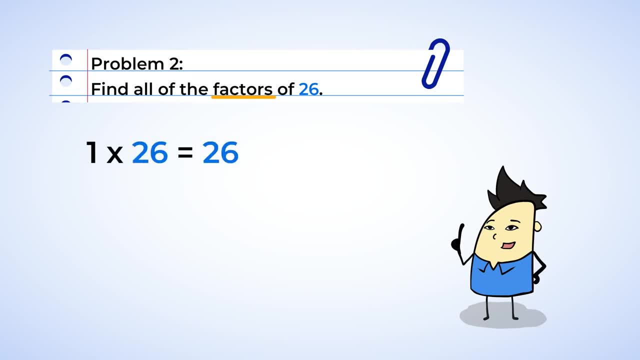 1. 1 multiplied by 2. 26 is 26.. Good, Next we can check 2.. Yeah, 2 multiplied by 13 is also 26.. Now we can move on to 3.. Um, no, 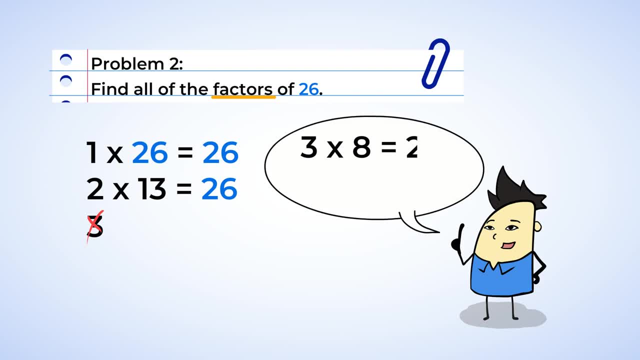 3 is not a factor, because 3 times 8 is 24.. And 3 times 9 is 27.. Okay, let's try 4.. No, not 4, because 4 times 6 is 27.. 4 times 7 is 24.. 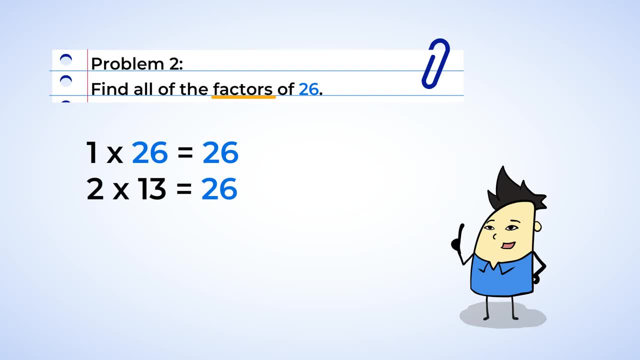 And 4 times 7 is 28.. Okay, Wow, as we continue to go through the numbers after 2,, there are no other factors until we get all the way up to 13.. Okay, so the factors of 26 are 1,, 2,, 13, and 26.. 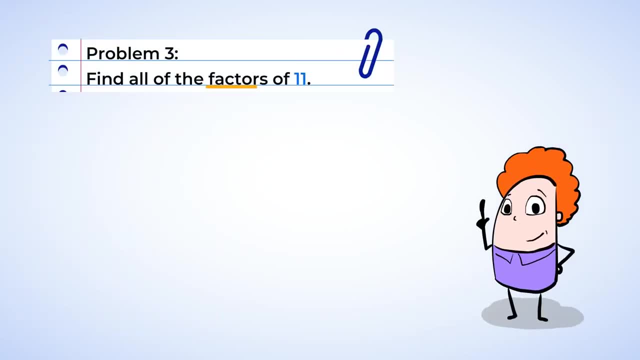 All right, Let's find the factors of 11.. Huh, Ooh, I remember Start with 1.. 1 multiplied by 11 is 11.. Okay, now let's try 2.. Nope, not a factor, since 11 is not an even number. 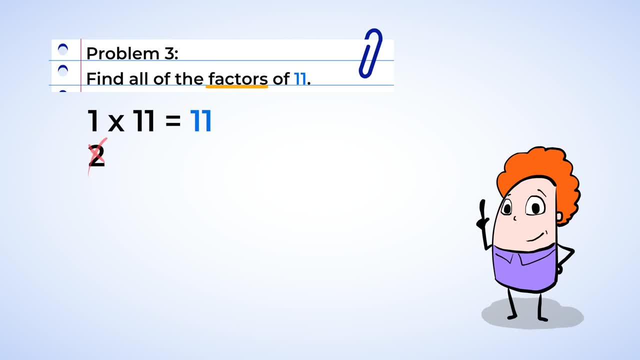 Okay, 3.. 3,, 6,, 9,, 12.. No, not 3.. Move up onto 4.. Moving onto 4.. No 5?, No 6?, Uh-uh, 6?. 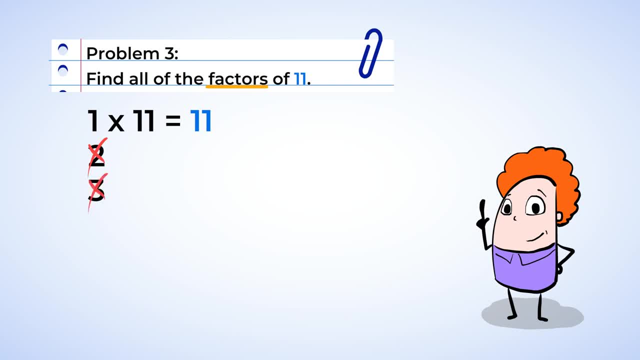 No 5? No 6?? Uh-uh, 5? No 6? No 5? No 6?? Huh, It looks like 11 only has the factors of 1 and 11.. 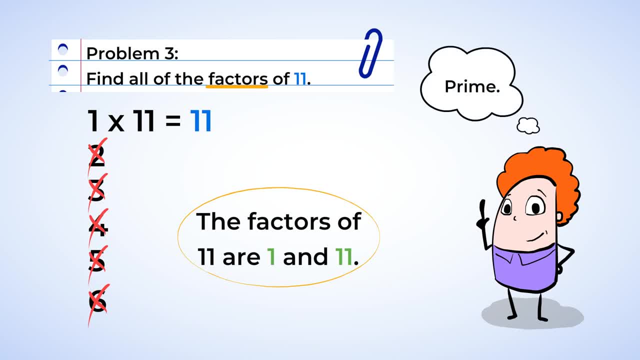 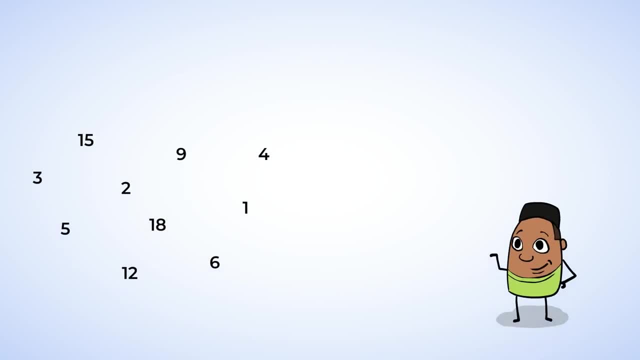 Ah, that means it's a prime number and the factors of 11 are only 1 and 11.. Whoa, look at all those numbers. Which of the following numbers are factors of 36?? Okay, the only way to get this done is to organize them to check if they are factors. 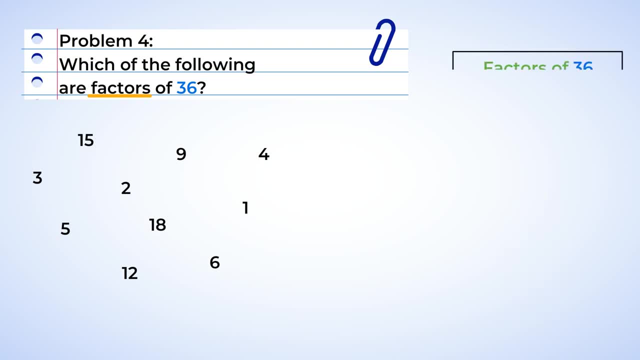 What if they are factors, by making two lists: Factors and not factors. Okay, let's get started. We know that 1 is a factor, so let's move onto 2.. 2 multiplied by 18 is 36.. Yes, 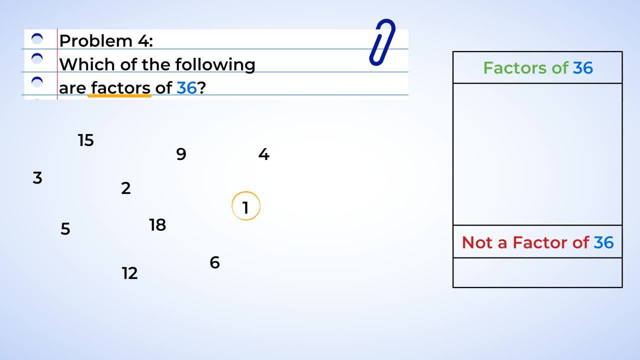 Oh, real quick. Don't forget about how multiplication and division are related. You can also think 36 divided by 2 is what number, but not 36.. If you add 36 to 36, what number do you think is 36?? 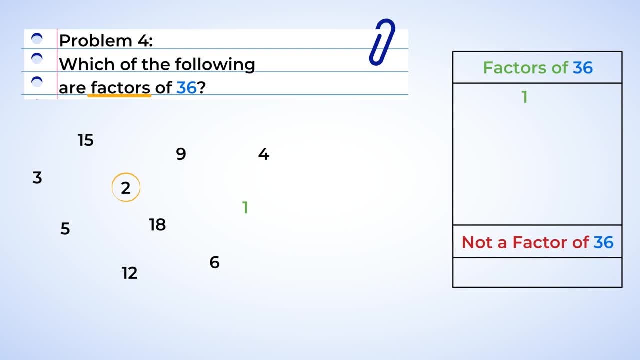 Oh, that's right. 36 divided by 2 is 36. Yes, 36.. So if we divide 36 by 36, we get 36.. 36 divided by 2 is 36. Yes, 36.. 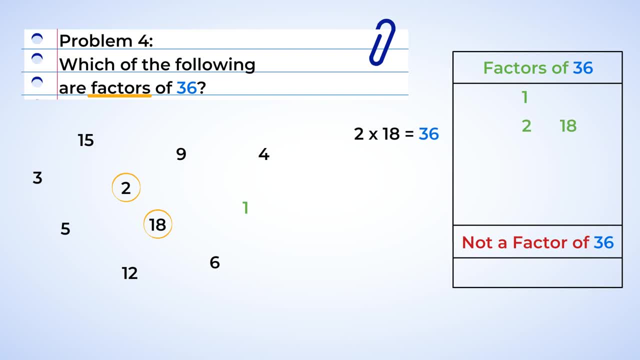 Okay, now let's get more into this. We can look at the number of numbers. We can also look at the number of numbers. We can look at the number of numbers Real quick. don't forget about how multiplication and division are related. 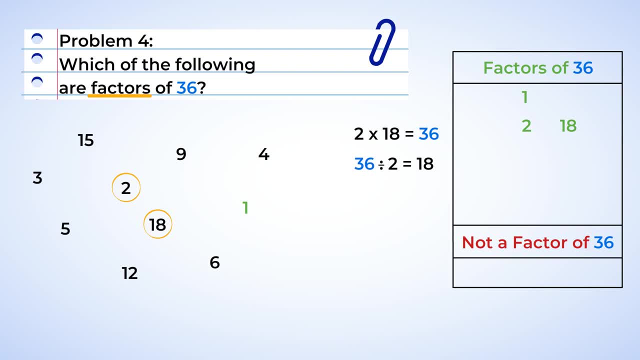 You can also think: 36 divided by 2 is what number? to find 18.. All right, so now we have that both 2 and 18 are factors. Okay, next is 3.. 3 multiplied by what is 36?? 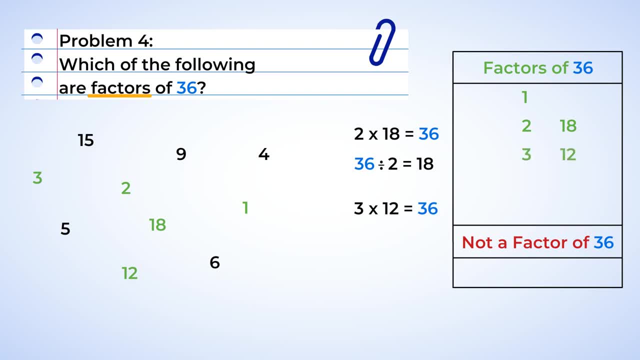 12.. Okay, we found two more factors. We're going to get good at this. Next is 4.. Um, ah, 4 multiplied by 9 is 36.. Okay, that's two more factors that have been found. 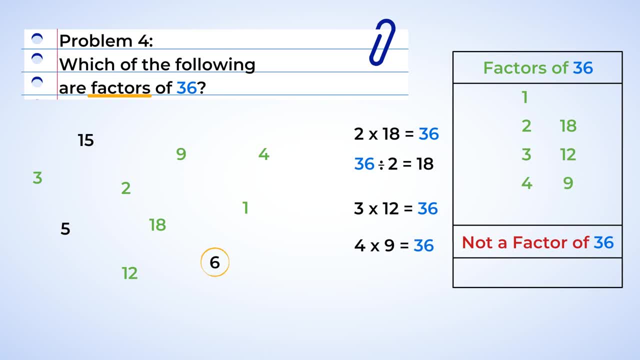 Next we can check 6.. 6 times 6 is 36.. Oh, another factor found. Aha, looks like we're starting to loop back up. So we have found all the factors And this means that 5 and 15 are not factors. 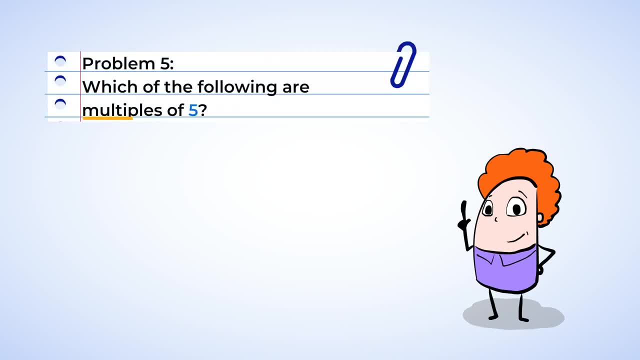 Okay, the last problem: We need to find the multiples of 5.. Well, that shouldn't be too tough. We can just skip count by 5.. So let's circle the numbers that are multiples of 5.. Okay, so we are starting with 5..